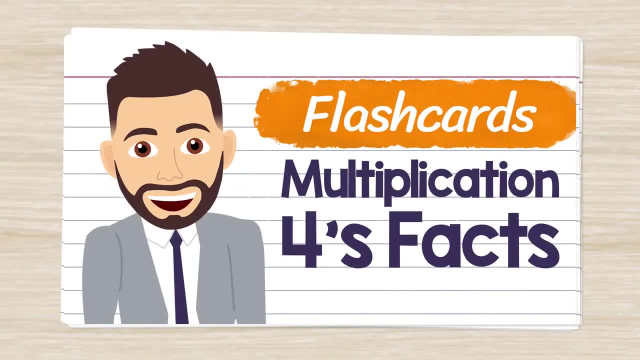 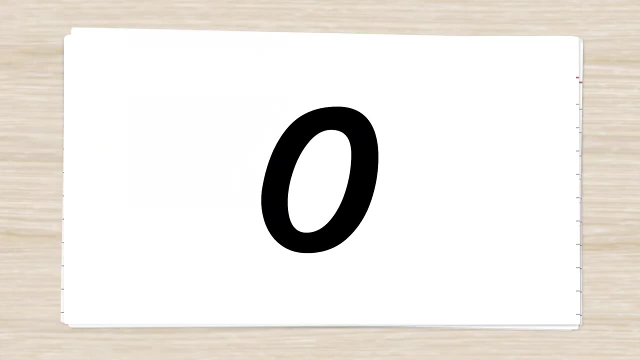 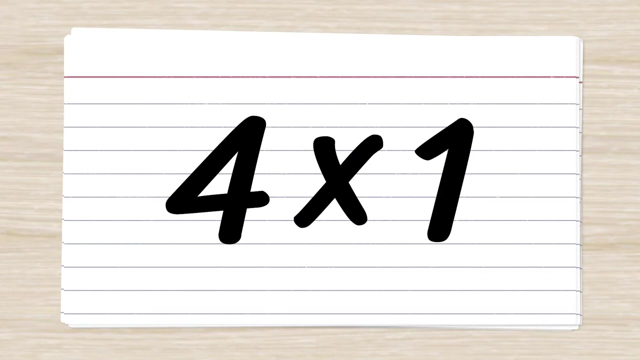 Welcome to Multiplication Flashcards with Mr J, And in this video we're going to go through the fours multiplication facts. So I hope you're ready, Let's get started. Four times zero, zero. Four times one. four, Four times two. 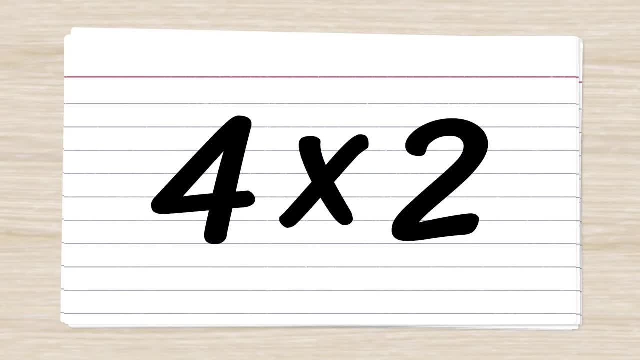 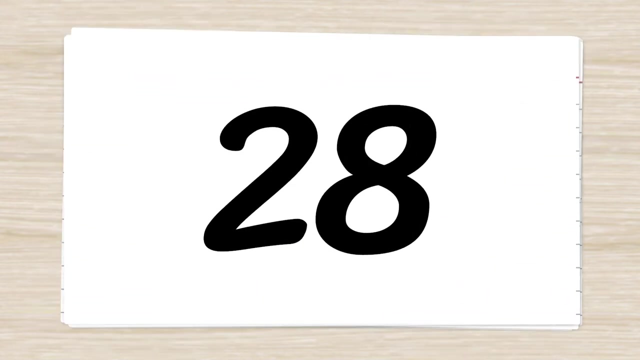 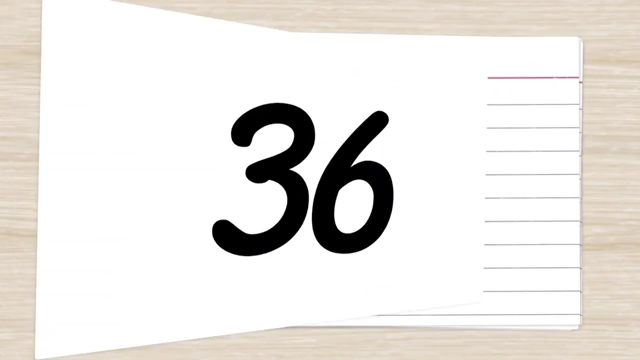 eight, Four times three. twelve, Four times four. Sixteen, Four times five. twenty Sixteen, Twenty, Twenty, Four times six. twenty-four, Four times seven. twenty-eight, Four times eight. thirty-two, Four times nine, thirty-six. 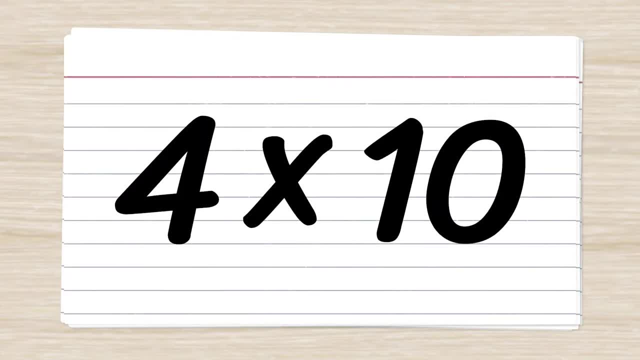 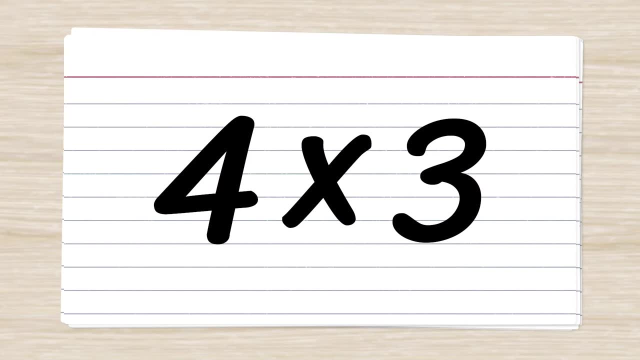 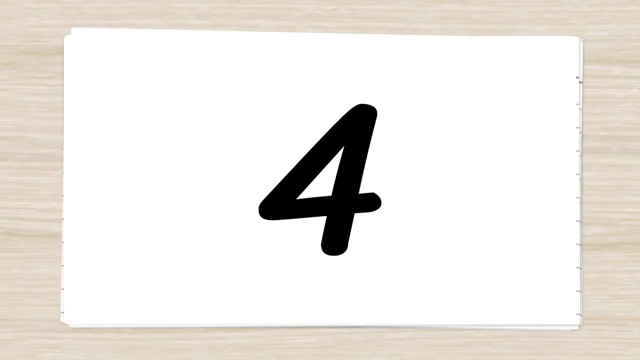 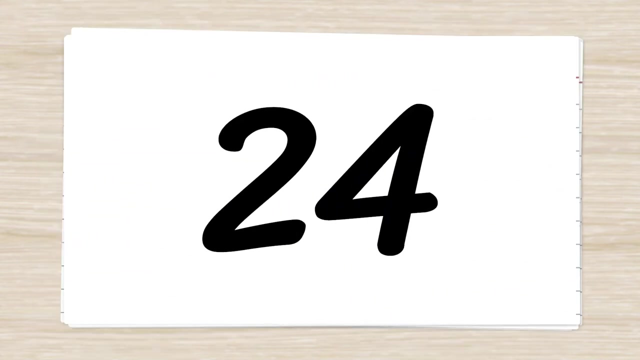 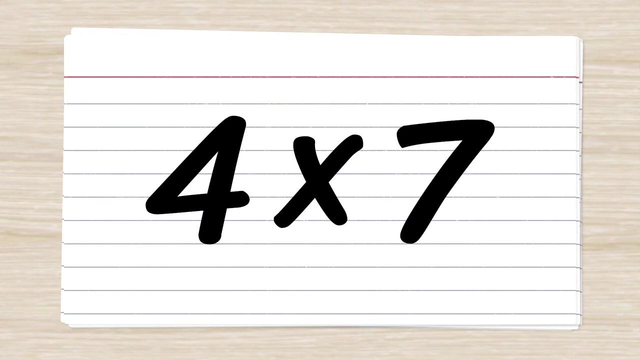 Four times ten. forty, Four times three. twelve, Four times five. twenty Four times one. four Four times four. sixteen, Four times six. twenty-four, Four times seven. Twenty-eight, Four times two, eight, Four times eight, thirty-two.